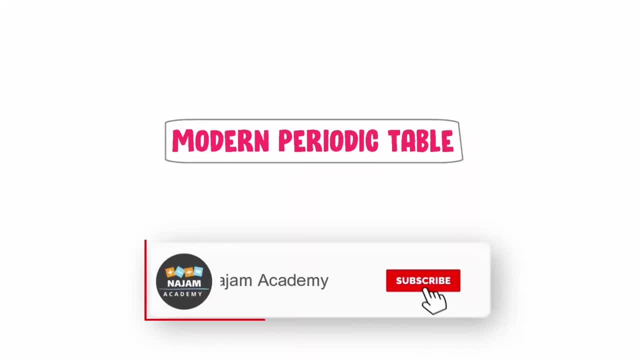 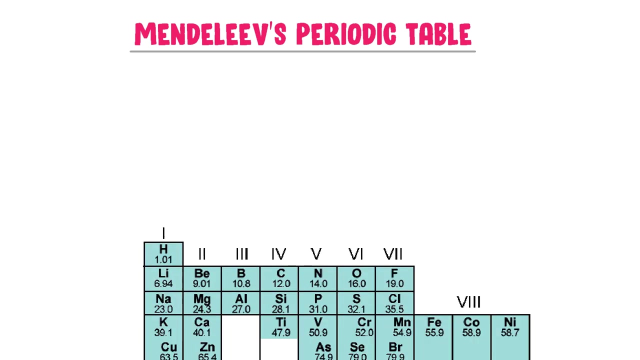 Modern Periodic Table. Before starting the lecture, click on the subscribe button and get access to our hundred of unique and simple lectures for free. Firstly, let me quickly revive the Mendeleev's Periodic Table, which we have learned in the previous lecture. We know that in the Mendeleev's Periodic Table, elements are arranged on the 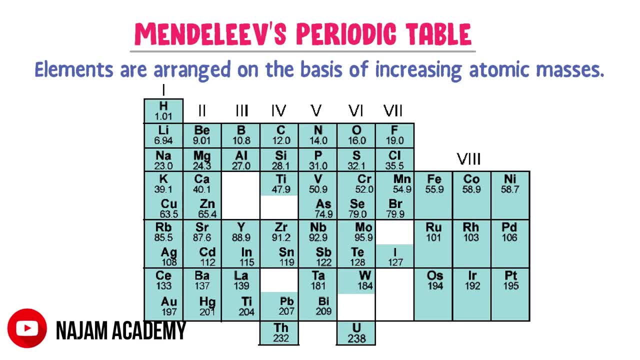 basis of increasing atomic masses. For example, the atomic mass of hydrogen is 1.01, the atomic mass of lithium is 6.94.. So Mendeleev Baba firstly placed hydrogen, secondly he placed lithium and thirdly he placed beryllium. Thus note it down that in the Mendeleev's Periodic Table, 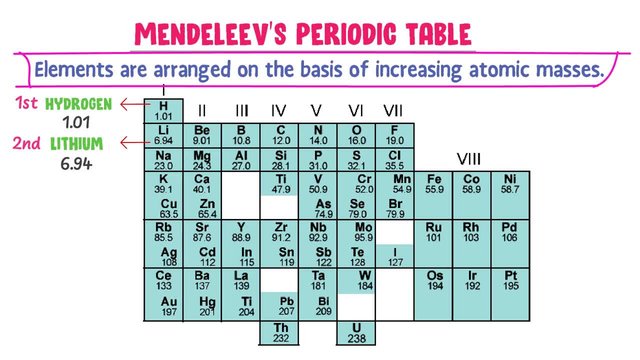 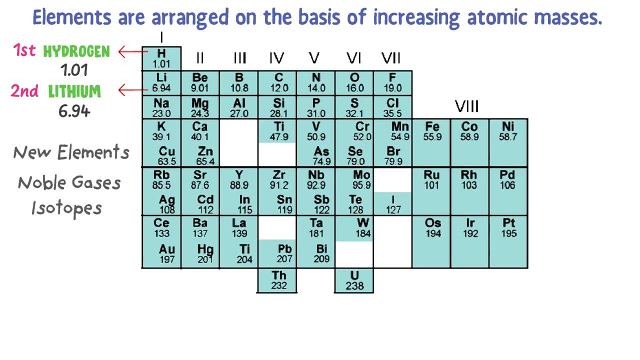 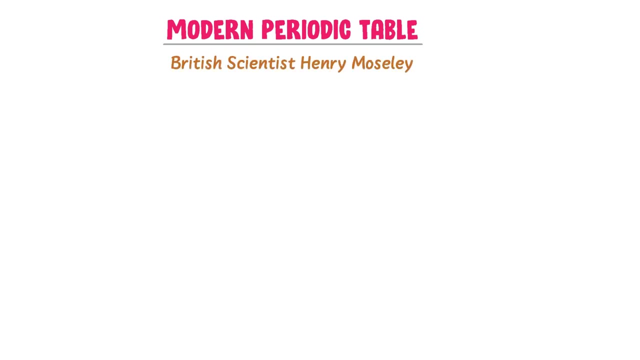 elements are arranged on the basis of increasing atomic masses. Later, when new elements were discovered, like noble gases or isotopes of different elements, it was difficult to place them in the Mendeleev's Periodic Table. So then scientists formed Modern Periodic Table. It was British scientist, Henry Moseley, who formed the Modern Periodic. 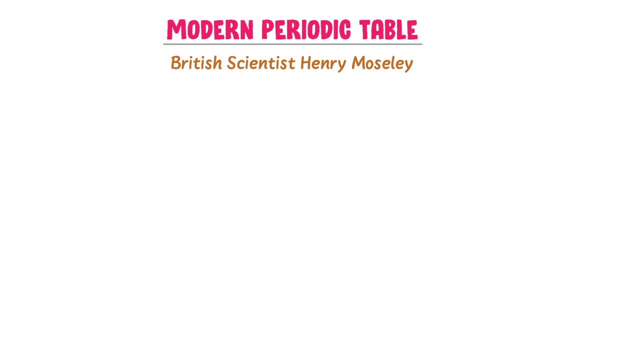 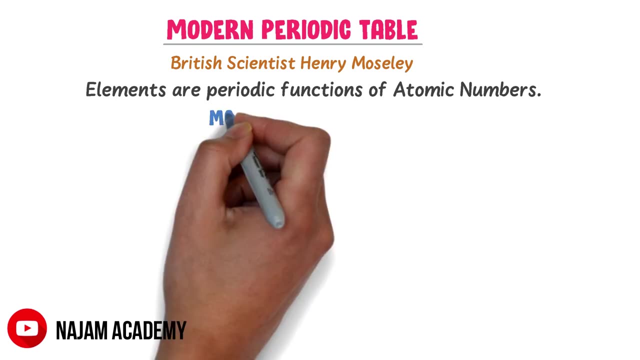 Table. He found something very interesting. He observed that elements are a periodic function of atomic numbers. He found that elements are periodic functions of atomic numbers. He called this as a Modern Periodic Law, which you will learn in this lecture. For example, 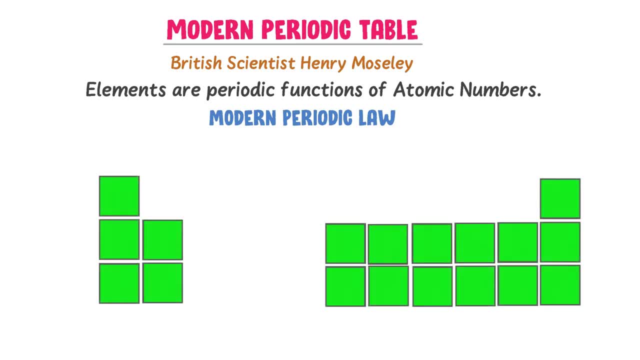 consider first 18 elements of the Modern Periodic Table. Now Moseley Baba placed elements according to increasing atomic numbers. Atomic number means the total number of protons present in an atom. The atomic number of hydrogen is 1, so he placed it as the first element of the Modern Periodic. 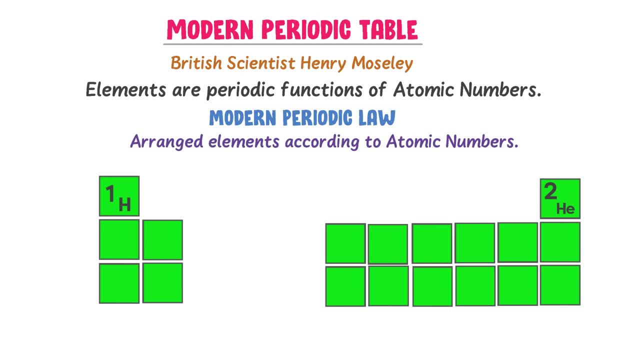 Table. The atomic number of helium is 2,, so he placed it as the second element. The atomic number of lithium is 3,, so he placed it as the third element. The atomic number of beryllium is 4, so he placed it as the fourth element. Hence, by this way, he placed elements in the Modern Periodic. 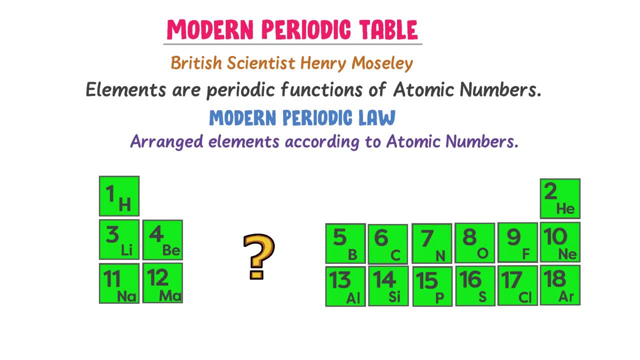 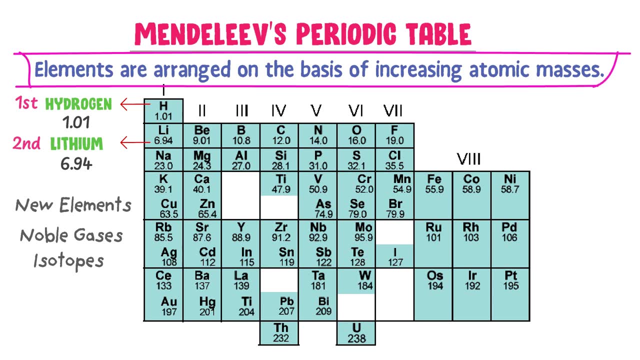 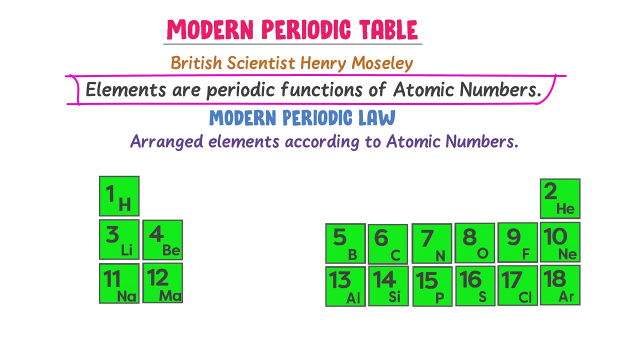 Table. Now, what is the main difference between Mendeleev's Periodic Table and Modern Periodic Table? Well, Mendeleev Baba arranged elements on the basis of increasing atomic masses. So in the Modern Periodic Table, elements are arranged on the basis of increasing atomic numbers. 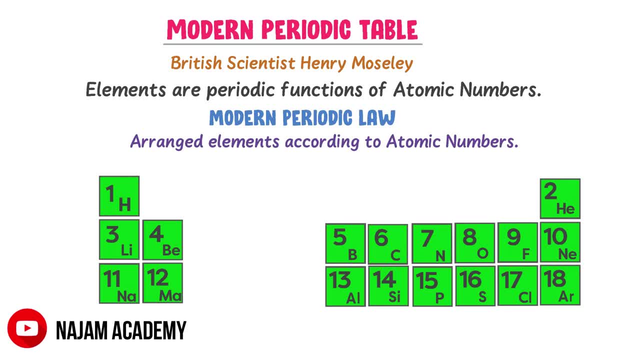 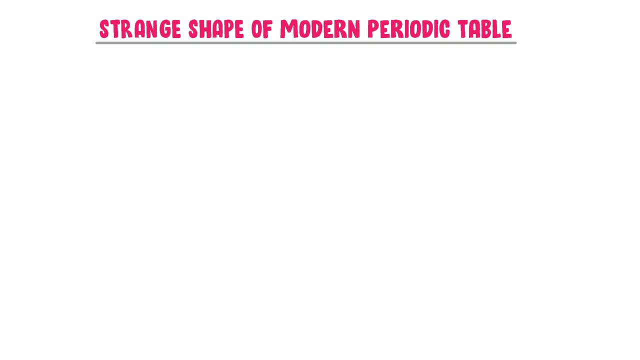 Also, we will study some other parameters of Modern Periodic Table, For instance, why Moseley Baba didn't place helium just after hydrogen and placed it here, Or why we have such a strange shape of Modern Periodic Table. Well, Moseley Baba ensured 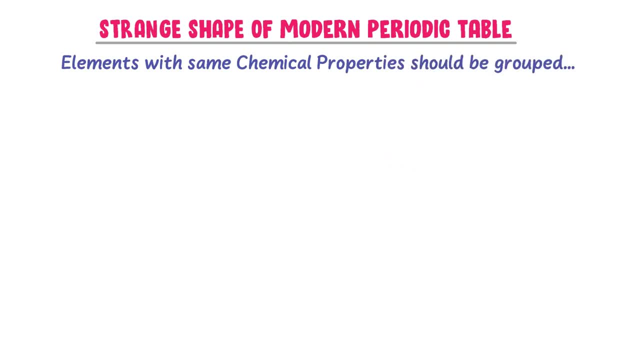 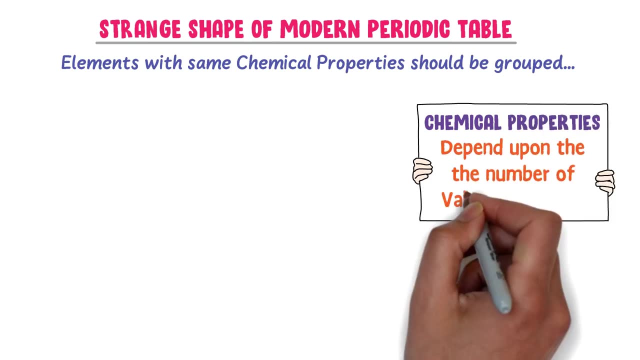 that elements with same chemical properties should be placed together in one group. Note it down that chemical properties depends upon the number of electrons and valence shell. For example, consider the group 1 elements like hydrogen, lithium and sodium. The atomic number. 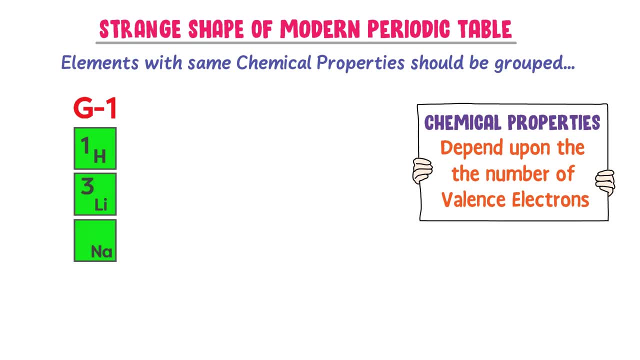 of hydrogen is 1,, the atomic number of lithium is 3, and the atomic number of sodium is 11.. We know that the atomic number is equal to the total number of protons or the total number of electrons, So the electronic configuration of hydrogen is one. 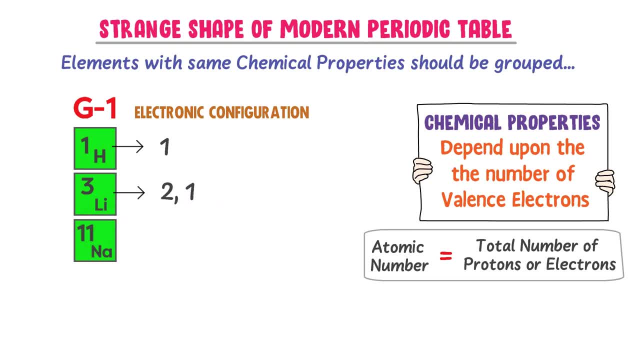 the electronic configuration of lithium is 2 comma 1, and the electronic configuration of sodium is 2 comma 8 comma 1.. We can see that these three elements have same number of electrons, or one electron and the outermost shell, So they also have same chemical properties. 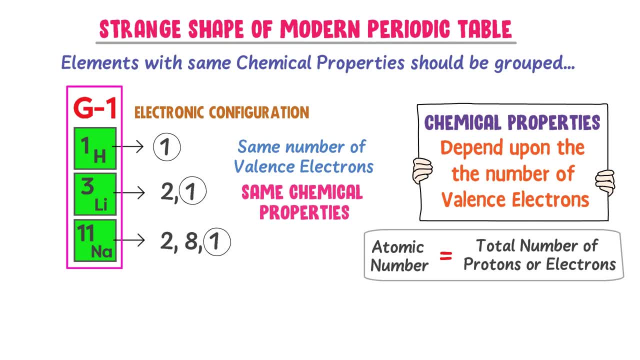 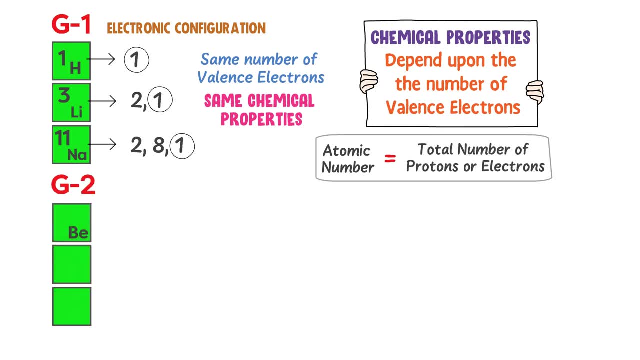 Thus Mosley-Baba placed these three elements in the same group, our first group. Secondly, consider the group two elements like beryllium, magnesium and calcium. The atomic number of beryllium is 4, the atomic number of magnesium is 12 and the atomic number 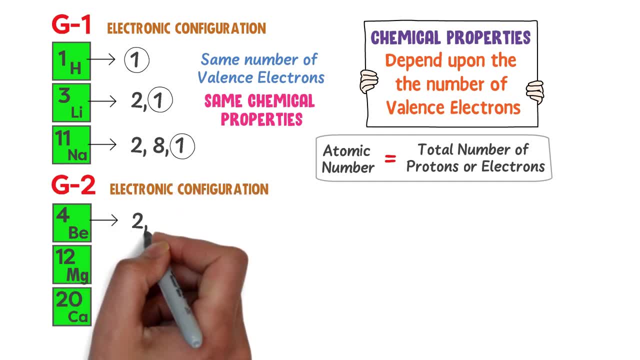 of calcium is 20.. The electronic configuration of magnesium is 2,8,2 and the electronic configuration of calcium is 2,8,8,2.. We can see that these three elements have same number of electrons: R2 electron and. 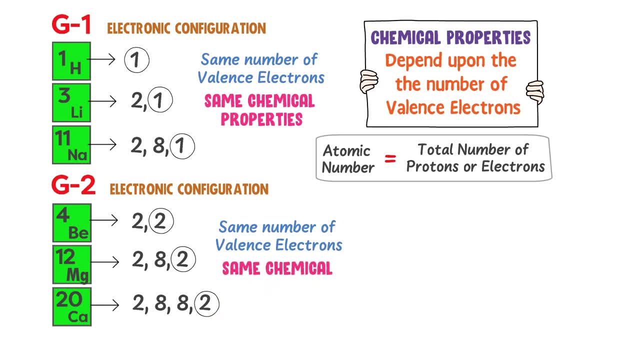 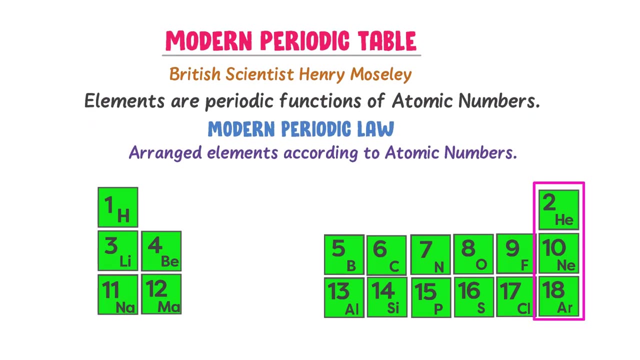 the outermost shells, so they also have same chemical properties. Thus Mosley-Baba placed these three elements in the same group. our second group, Similarly helium, is placed in this group because helium has same chemical properties as neon or argon has.